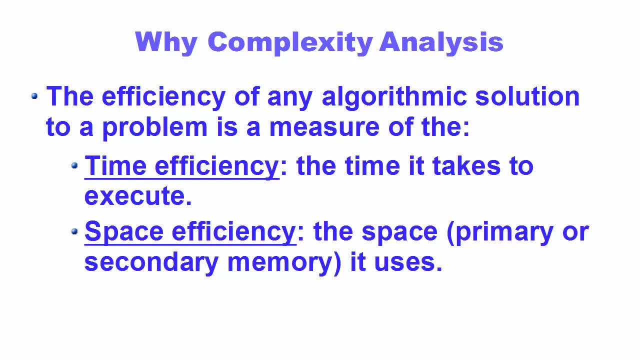 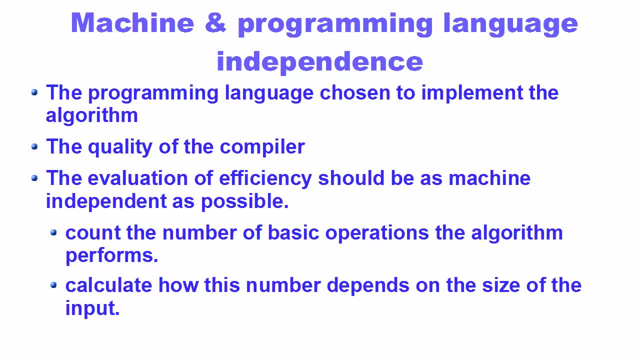 deals with the time. that means how much time an algorithm takes to execute. and space efficiency deals with the memory usage. that means how much space an algorithm take. Also, the evaluation of efficiency should be as machine independent as possible. It's not useful to measure how fast an algorithm runs if 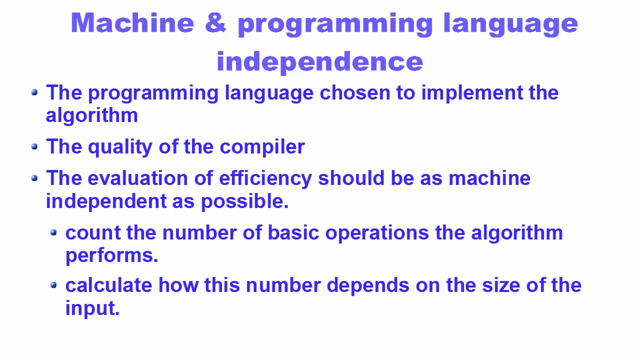 it depends on which particular computer or operating system or programming language or compiler or the kind of system which is needed. It's not useful to measure how fast an algorithm runs if it depends on which particular computer or operating system or programming language or compiler or the 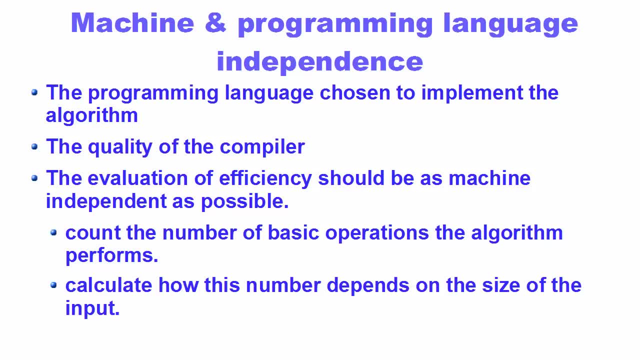 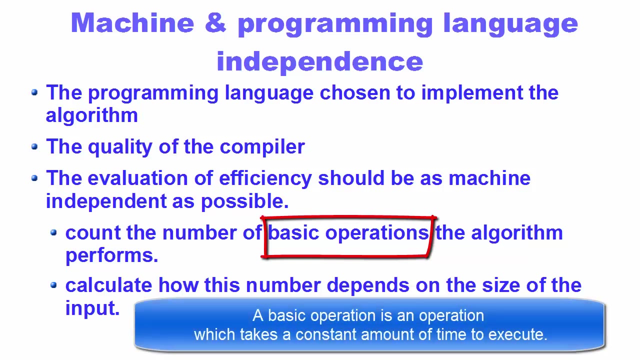 kind of inputs are used for the testing. Instead, to evaluate the efficiency of an algorithm, we count the number of basic operations the algorithm performs, and we also calculate how this number depends on the size of the input. Now, what is a basic operation? So a basic operation is an. 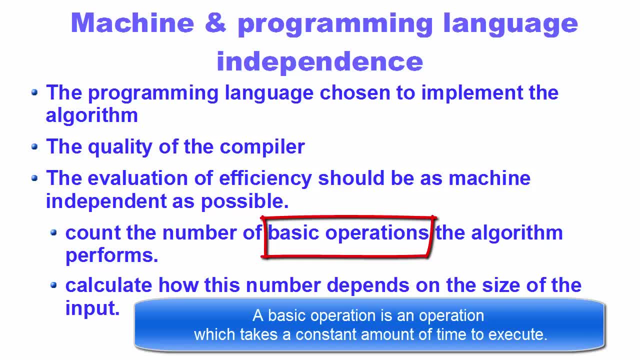 operation which takes a constant amount of time to execute. Hence the efficiency of an algorithm is the number of basic operations an algorithm performs. Now let me give you some examples of basic operations. So addition, subtraction, multiplication, memory access. when you return. 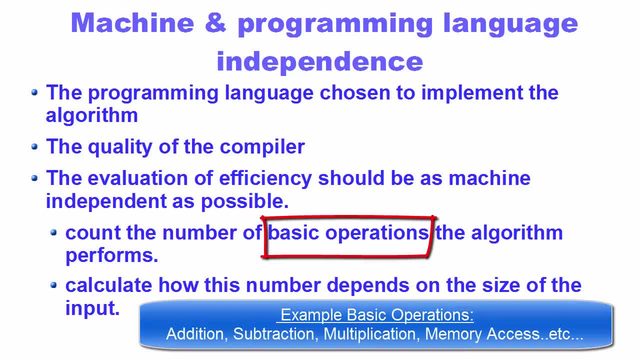 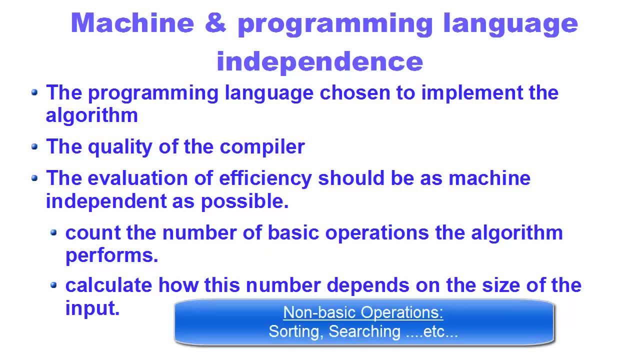 from a function. these are all basic operations. Now, what are non-basic operations? So operations like sorting of any big array or searching inside number of elements inside an array can be a non-basic operation. So in this course we are going to focus on the efficiency with respect to time, So we 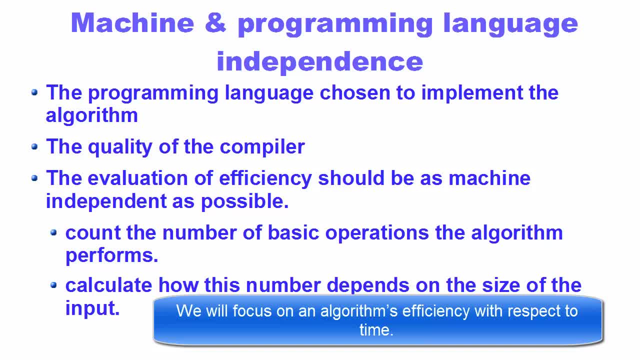 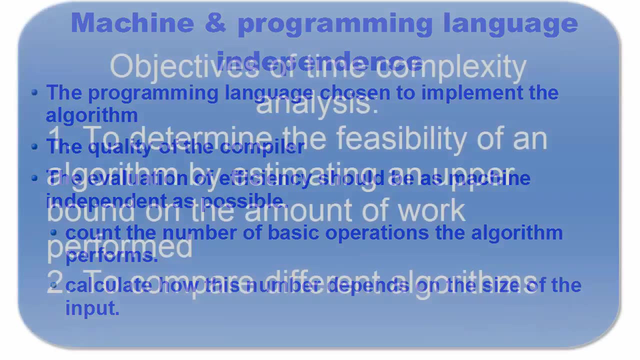 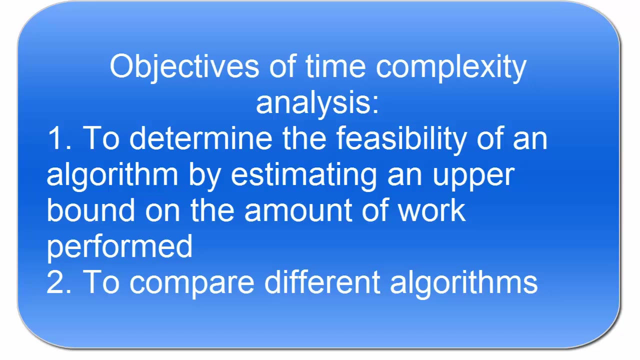 are going to speak about the time complexity and we are going to skip the space complexity, because often we use time complexity over space complexity to find out the efficiency of an algorithm. Now, the objective of time complexity analysis is to determine the feasibility of algorithm by estimating. 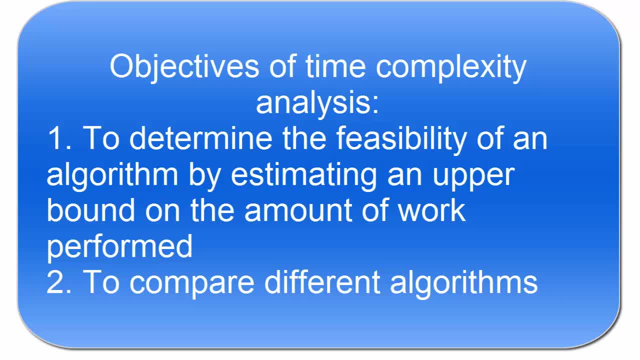 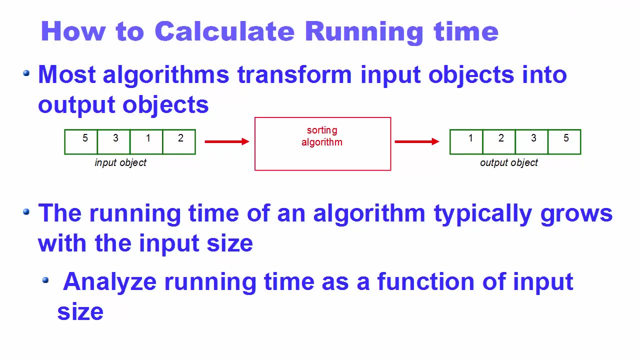 the upper bound of the amount of work performed and to compare different algorithms before deciding which algorithm is the best for solving a particular problem. Now, how to calculate the running time or how to find out the time complexity. So we all know that most algorithms transforms the input objects. 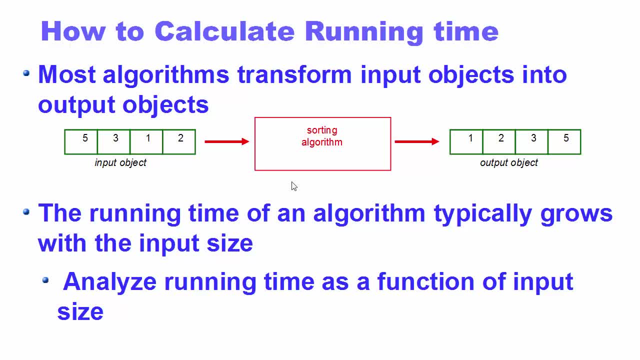 into the output objects. So, as an example, let's say we have been given an unsorted array which we want to sort with the help of an algorithm, So our input will be an unsorted array and then we apply an algorithm to sort an unsorted array which we want to sort with the help of an algorithm. So our input will be an unsorted array and then we apply an algorithm to sort. 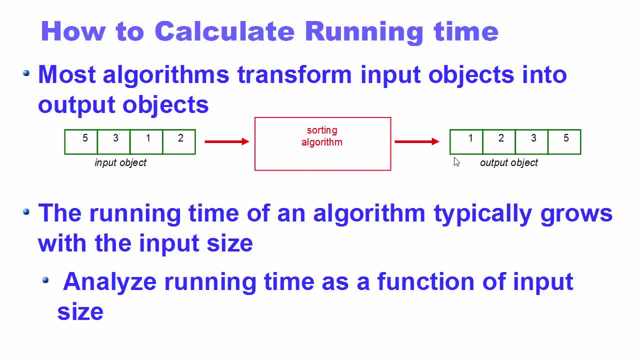 this array and, as a result, we get the sorted array in this form. Now it's important to note here is that the running time of an algorithm typically grows with the input size. Now, as we can see here that this input is of four elements. but if you want to calculate the running time or the time complexity, 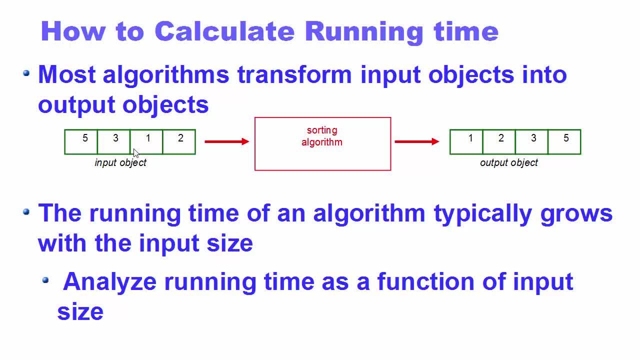 of an algorithm, we need to give a very large input to it and evaluate how this algorithm performs when we give a very large input to the algorithm. So generally we analyze running time as a function of input size, So how our running time behaves when we change the input size and we increase. 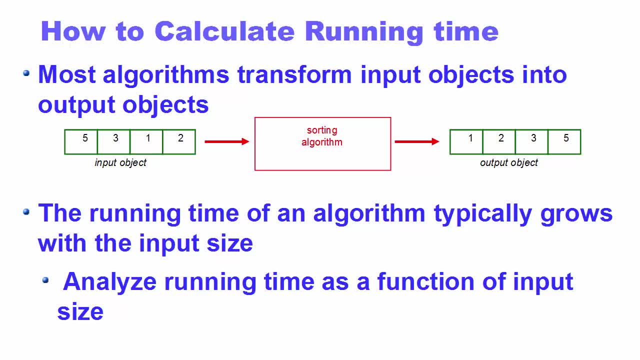 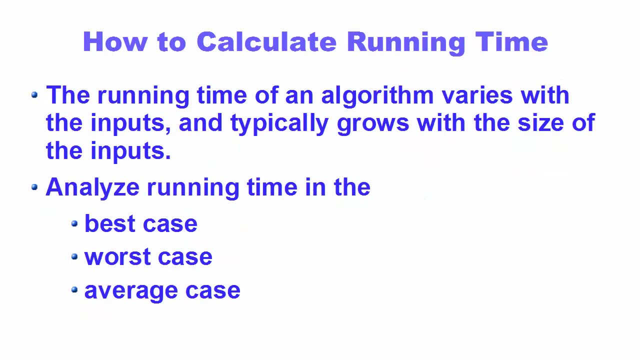 the size of our input and to evaluate an algorithm or to compare two different algorithms, we focus on their relative rate of growth with respect to the increase in the input size. Now, as I said, the running time of an algorithm varies with the inputs and typically it. 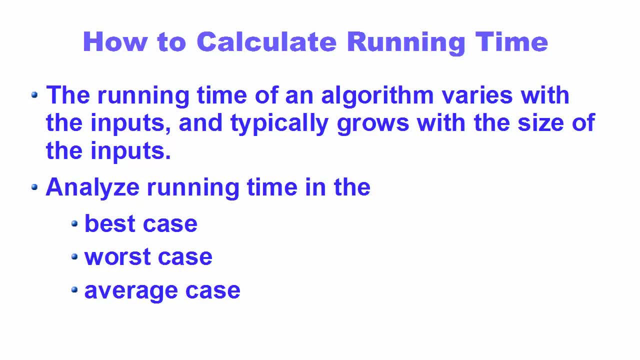 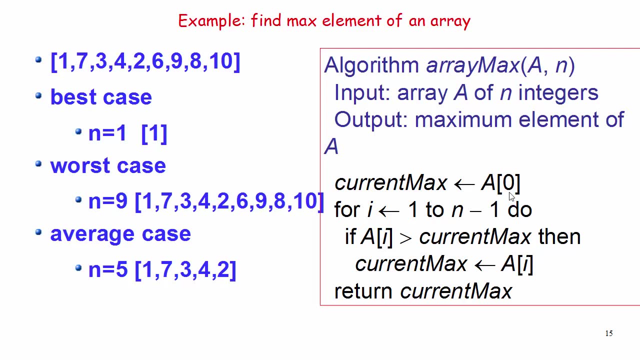 grows with the size of the inputs. Now we analyze the time in three different cases: The best case, the worst case and the average case. So let me explain you all these cases with an example. So on the right-hand side you can see I have a pseudo code. 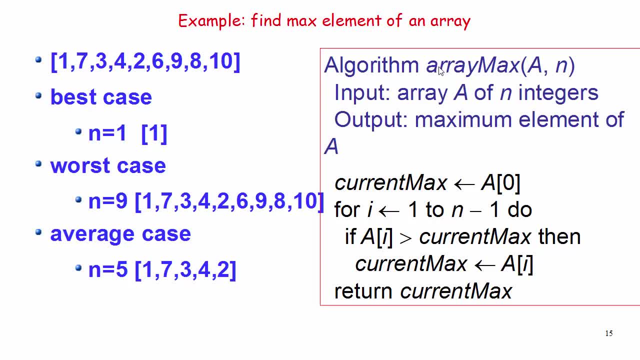 which contains a function which is called arrayMax. So we want to find out the maximum value inside an array. So here I have declared a pseudo code for a function, and the function name is arrayMax and the input which it takes is the array itself and the number of elements the array contains. 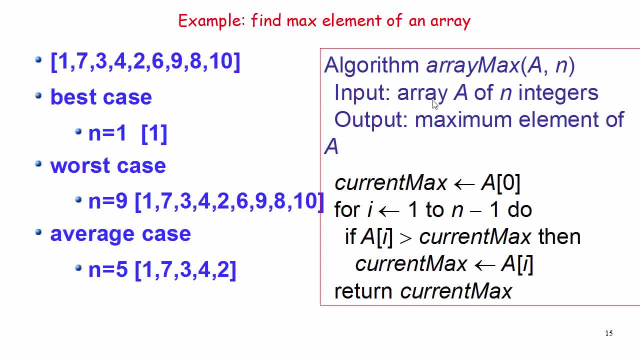 So here you can see the input arrayA of n integers and the output which we want is the maximum element value inside the arrayA. And let's say we write a very simple linear algorithm to calculate or find out the maximum value inside an array. So in this algorithm, first of all we just take or consider the 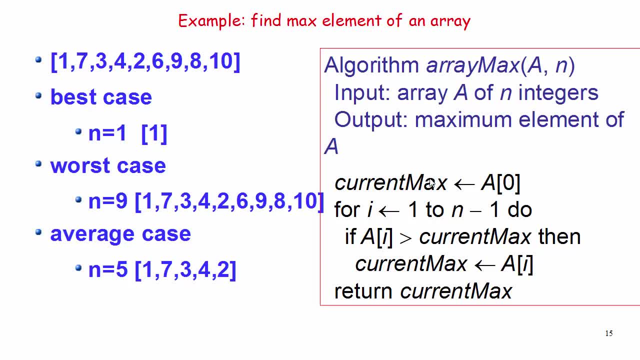 first value of an array, which is at index 0, as the maximum value, and then we iterate over the elements of an array one by one And inside the for loop. we compare each and every element of the array with the current maximum value which is taken for from the first element of an array, And if this value 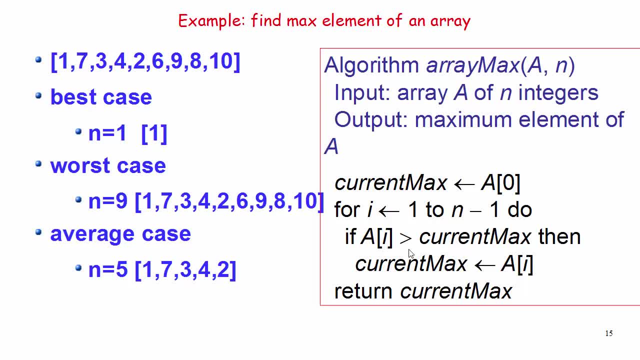 is greater than our current maximum value, then the maximum value of the array is greater than the current maximum value of the array. We are going to change the current maximum value to the new value and, in the end of the function, we are going to return the current maximum value using 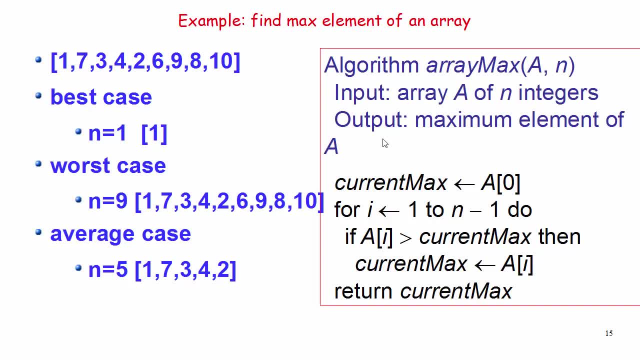 this function. So the inner working of the function right now is not very important. The important thing is the input which we are giving here. So let's say the maximum size of an array which we can provide inside this function is 9.. So let's say we can only provide the array of 9 elements inside this. 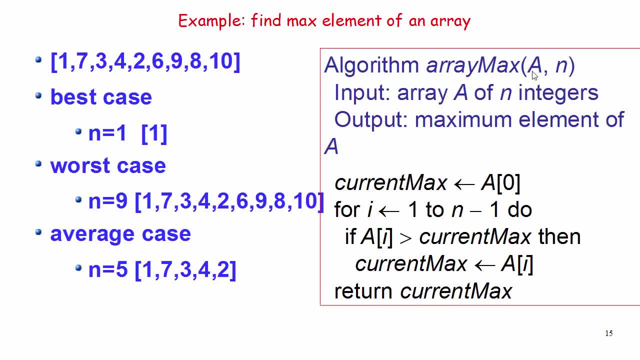 function, Then the worst case scenario in this case will be when we provide an array of 9 elements, Because this for loop has to iterate over all the 9 elements to find out the maximum value. Now the best case scenario will be when we pass an array of only one element. we cannot pass an array of zero element. that's why our best. 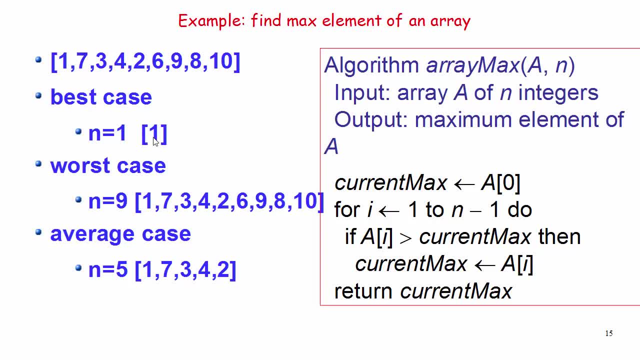 case scenario will be an array of element one, because it's going to take the least amount of time, because the for loop just have to iterate once to find out the maximum value, which is the value itself. and in the worst case scenario, you can see, because we can only provide nine elements. 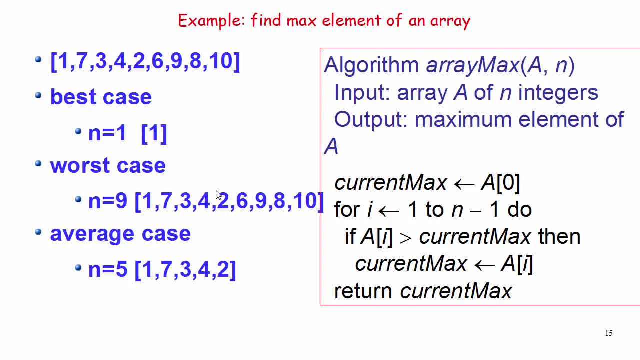 inside the array maximum. that means in this case it's going to take the most amount of time. i'm just taking this input as the hypothetical case to explain you the worst case scenario. so the worst case scenario is the maximum possible input you can give to an algorithm. 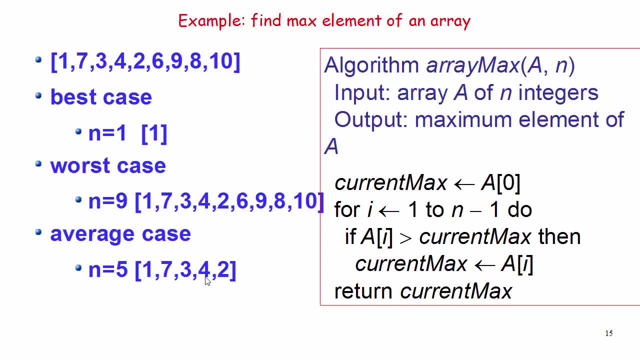 and the average case scenario will be in the middle of the best case and the worst case. That means in this example, an average case scenario will be an array of five elements. So in this case, the time taken by the algorithm to find out the maximum value will be in between the worst case and the best. 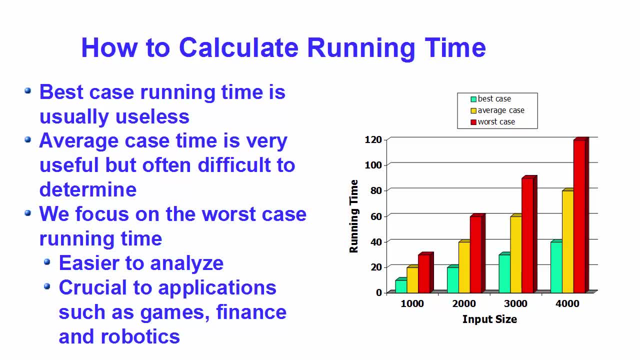 case, Now the best case. running time is usually useless because in real world it will never happen that a best input will be provided for your algorithm to find out the running time right. and the average case scenario is very useful, but it's often very difficult to determine. So 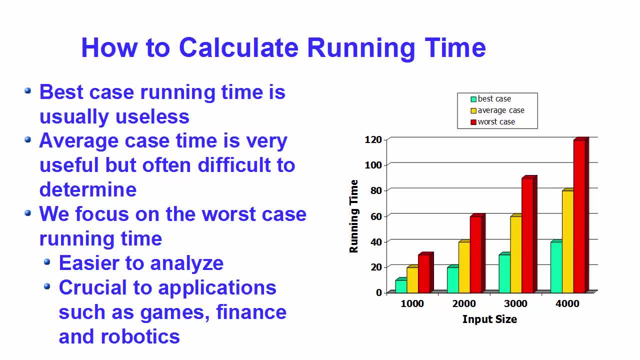 generally, we focus on the worst case scenario to calculate the running time because it's easier to analyze and it's crucial to find out the worst case running time in the applications like games or finance applications or robotics. So in those cases it's best to find out the worst case. 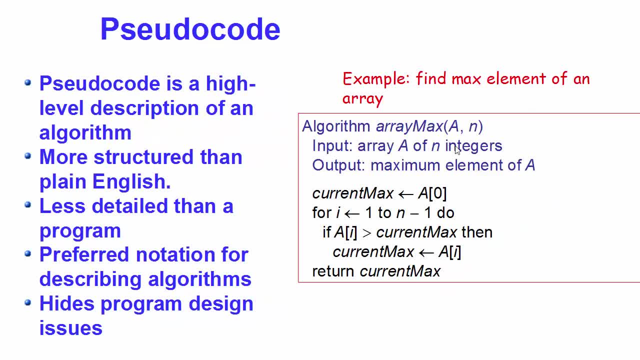 scenario. Now, in the last slide, I have shown you a pseudo code to just explain you how the best case, the worst case and the average case running time scenario works. So let me explain you what the best case running time scenario is and what the worst case running time scenario is.